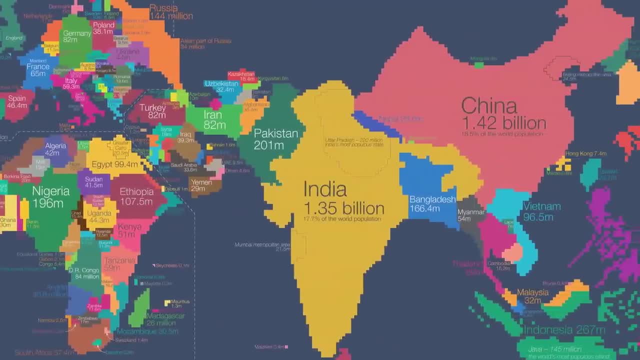 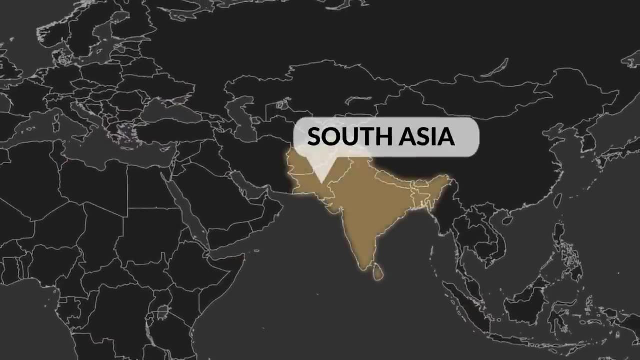 at this cartogram, which shows the different populations of each country in the world Today, we can see that there are four big regions that have over 2 thirds of the world's population living in them: South Asia, which consists of countries like India, Bangladesh and Sri. 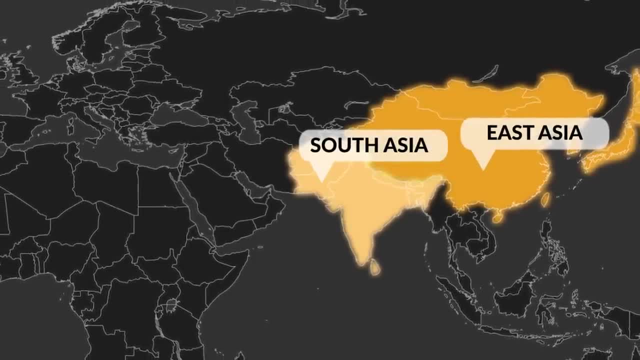 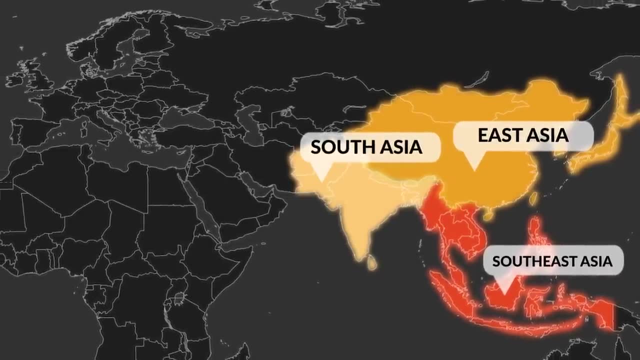 Lanka. East Asia, which is made up of countries like China, Japan and the Korean peninsula. Southeast Asia, which is made up of a variety of different countries, such as Thailand, the Philippines and Vietnam, just to name a few, And lastly, Europe, which, unlike the other regions, has people located. 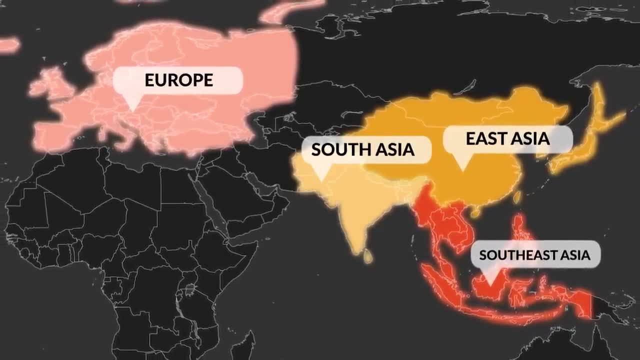 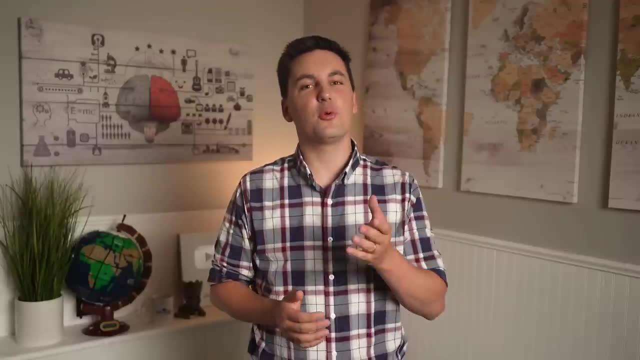 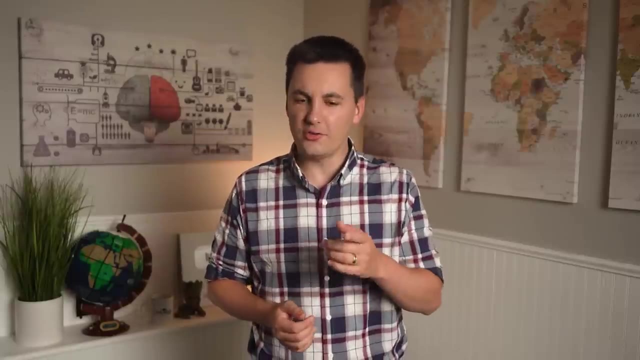 closer to natural resources instead of grouping around the rivers and oceans, which is particularly due to the industrial revolution and the location of raw resources. So, since each country has different populations and their populations are dispersed differently, it's hard for us to answer the question of: is the world overpopulated? In fact, maybe we should be asking: are certain? 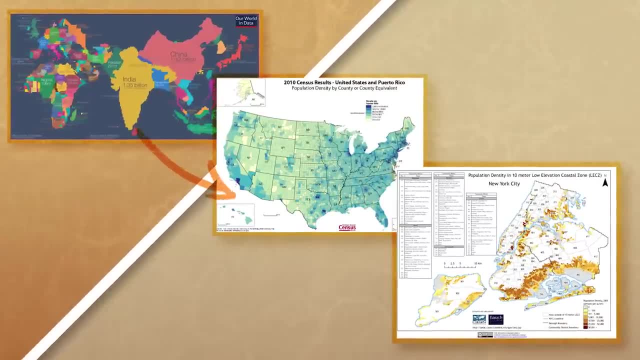 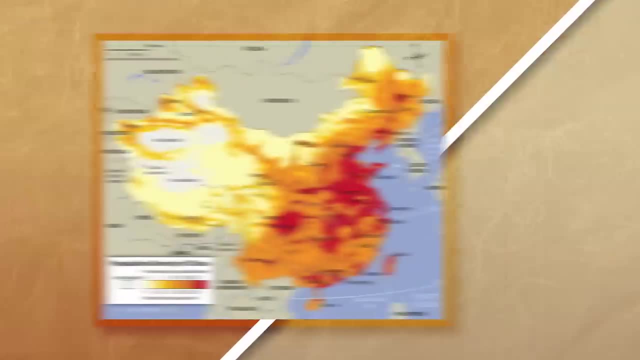 countries overpopulated. Well, if we change our scale from a global scale to a national scale or even a local scale, we can see that even this question becomes more difficult to answer. For example, when looking at China's population density, notice that the majority of the areas 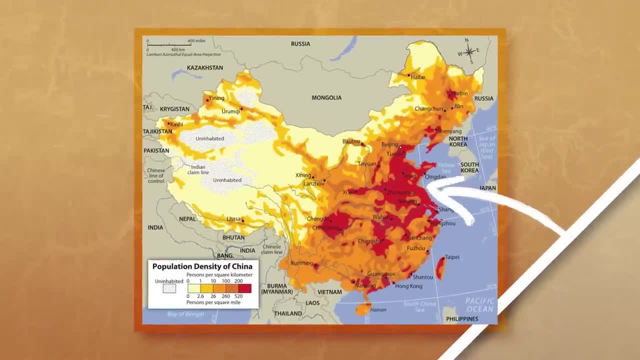 with a higher population density are near the coast of China or near China's river. In the case of China, the population density is lower than the coast of China. In the case of the coast of China, the population density is lower than the coast of China. In the case of. 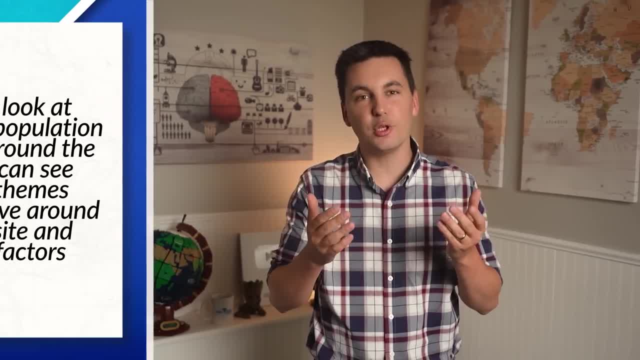 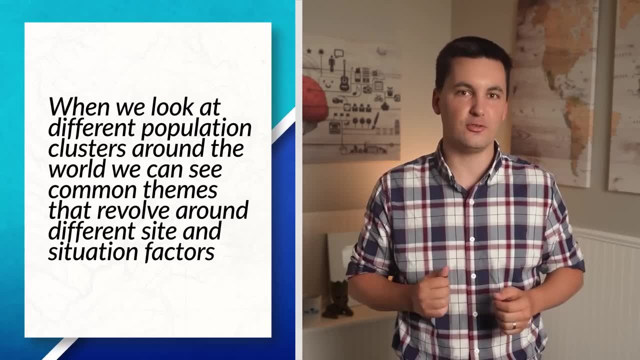 China, the population density is lower than the coast of China. In fact, if we look at different population clusters around the world, we can see common themes that revolve around the different site and situation factor. Throughout the world, we can see that people tend to settle by rivers. 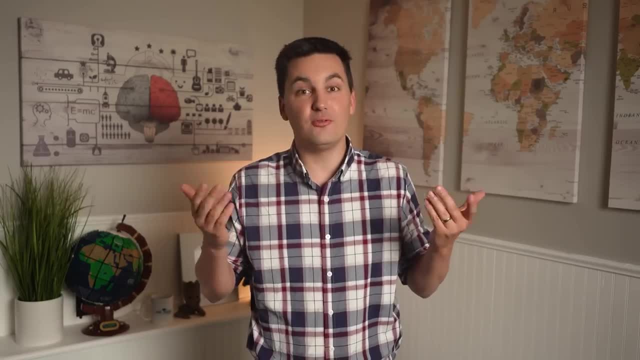 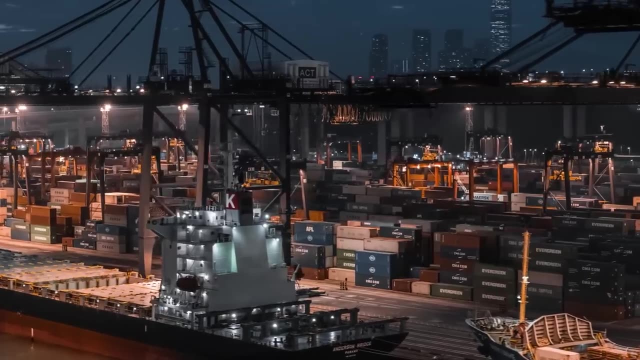 oceans, fresh water and fertile soil. This is because people need food and water to live. Plus, access to oceans and rivers that connect to other geographic areas allow places to participate in trade and commerce with places around the world. We can see that people also gravitate towards air. 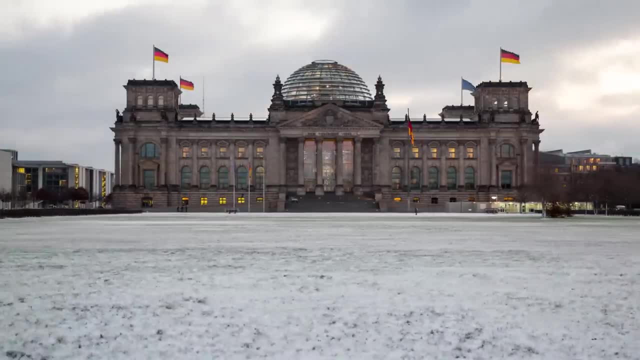 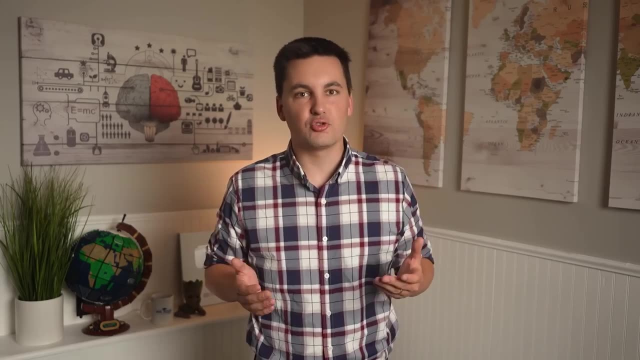 areas with economic opportunities, political stability, desired cultural preferences, or may live in a place due to historical events that created the settlement. So even when looking at a country, it can be hard for us to tell if the country overall is overpopulated because people 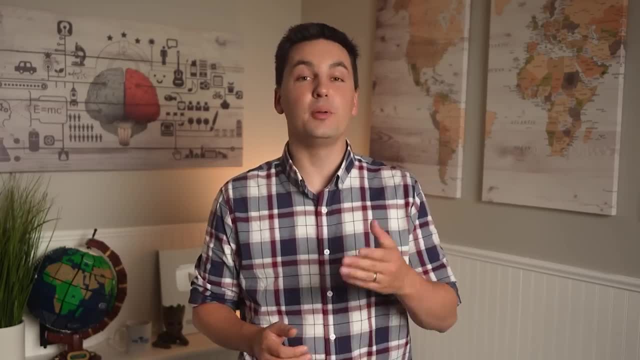 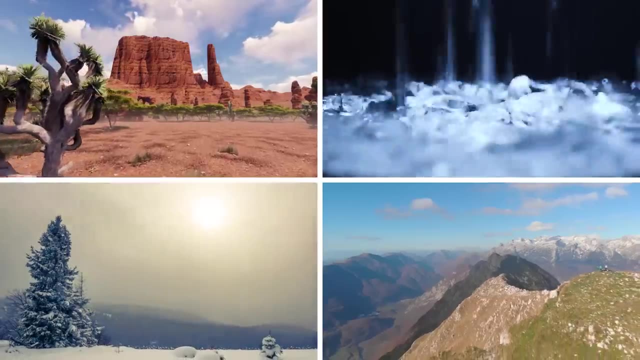 will be dispersed differently in each country. Now, since we talked about places where people want to live, we also need to talk about places where people generally do not want to live. These are often places that are too dry, too wet, too cold or too high. Areas that are too dry make it. 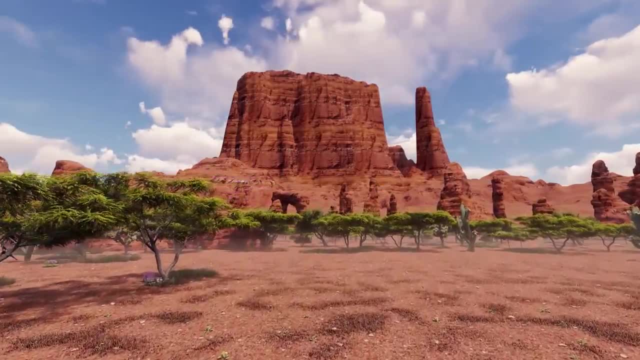 difficult to grow. So if you're in a place that's too dry, too wet, too cold or too high, you can't grow crops, which does not help create a stable society. A similar problem actually exists for places that are too wet: Soil becomes oversaturated, which ends up killing the crops. 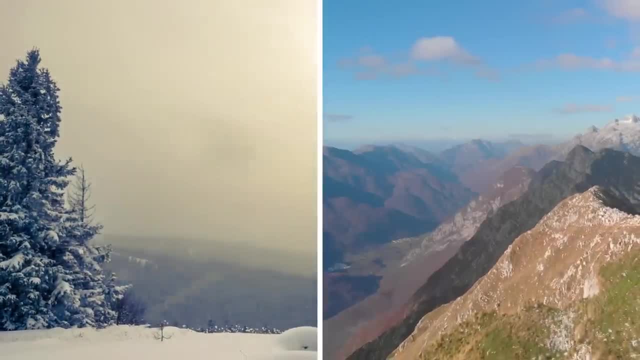 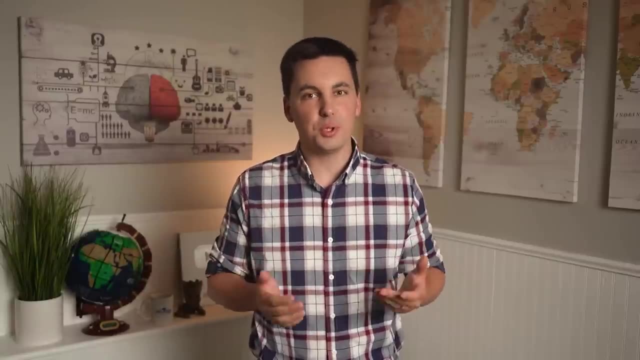 Places that are too cold or too high are often difficult to live in and do not provide the adequate resources needed for a society to flourish. Today, thanks to advancements in technology, we can see that people live in places where it was never possible to have permanent 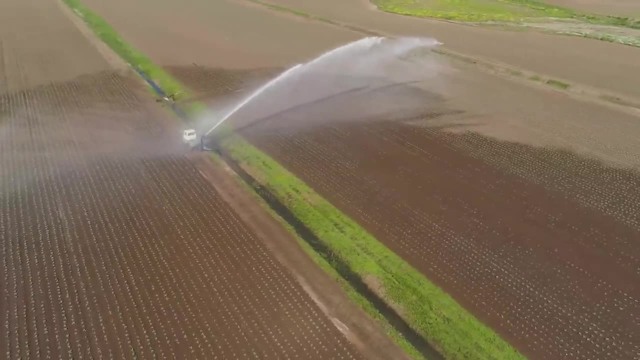 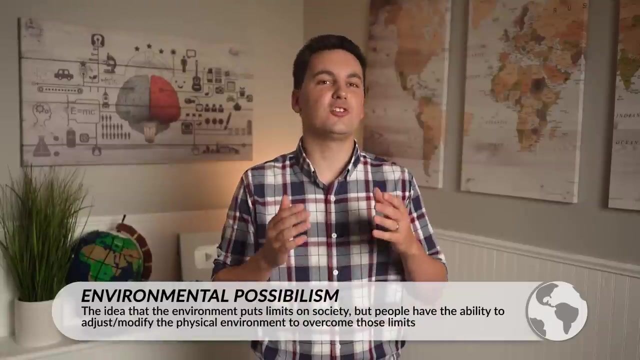 settlements before. This ability for us to modify and change our environment, to make less hospitable areas more hospitable, is known as environmental possibleism, a concept we reviewed from Unit 1.. So we can see that, depending on the different site and situation, 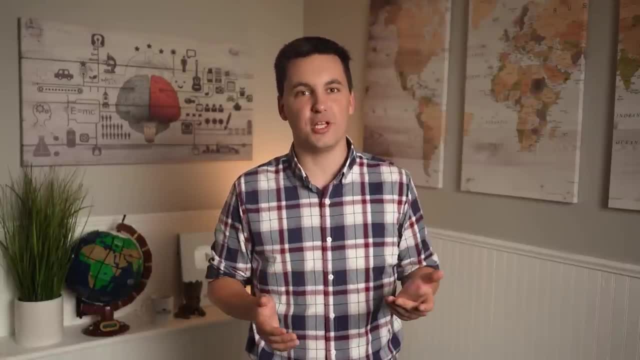 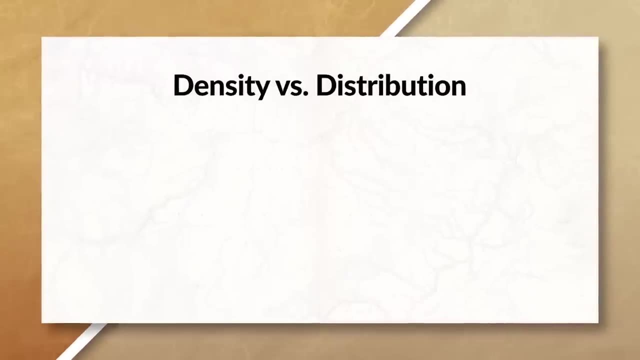 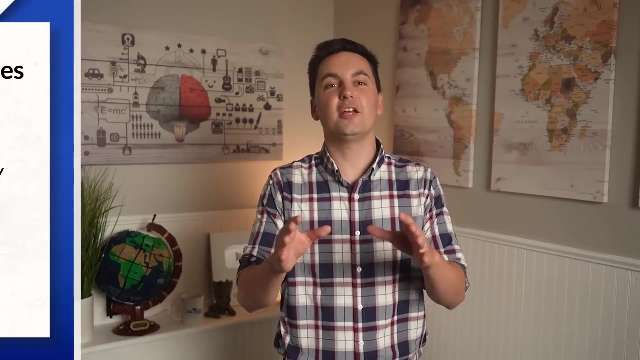 factors a place may be more likely to have a higher population density, while other factors may promote a lower population density. Remember, population density is different from population distribution. Population density is referring to the number of people in an area, while population distribution is the spread of people in an area. When looking at density, we can see that there. 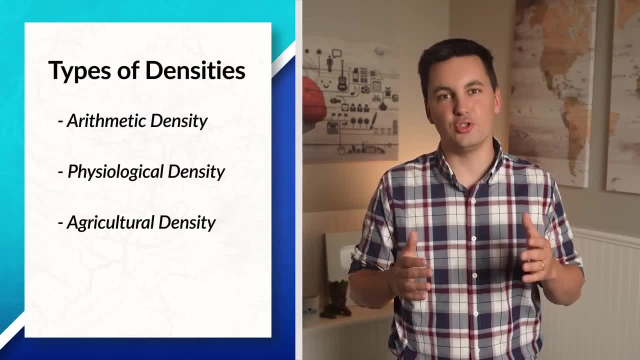 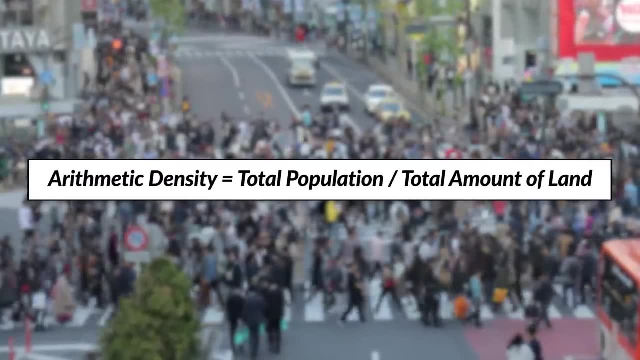 are three different types of density that you'll see in api- human geography. The first density is the arithmetic density. To find this density, we need to find the number of people in an area. To find this density, we are going to take our total population and divide by the amount of. 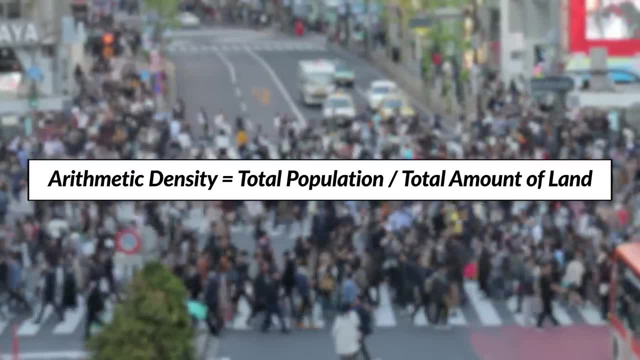 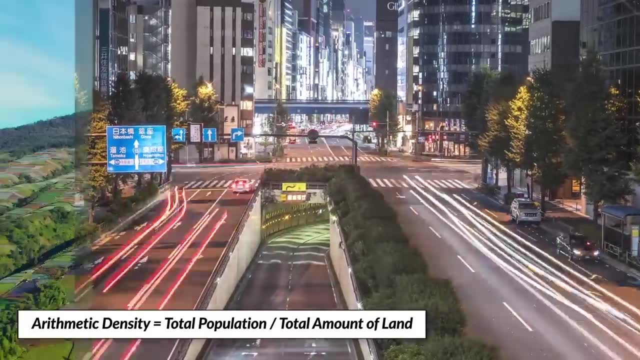 land. This is one of the easiest densities to find. This density shows us how many people are living on each unit of land. If this number is really high, it means that there are more people living near each other. If the number is a smaller number, it shows that there are fewer people. 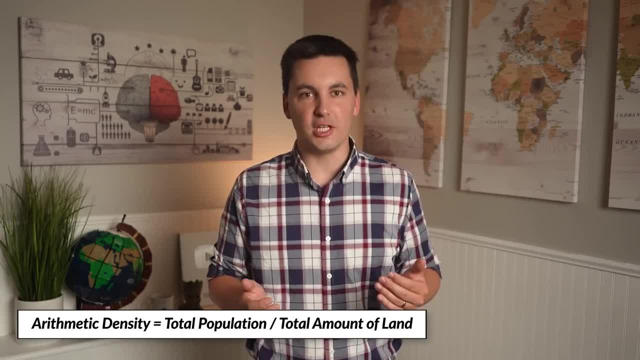 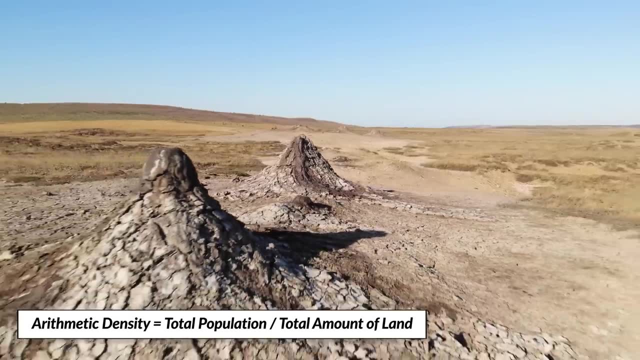 living on each unit of land. One thing to remember when looking at this density is, when we say that we're dividing by the total amount of land, we mean the entire landmass, which could include land that is not inhabitable or land that currently has no one living on it. So 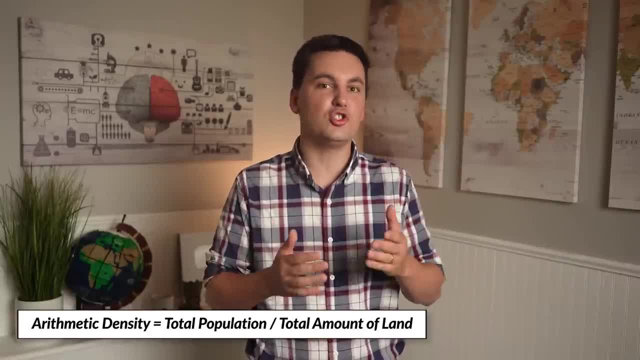 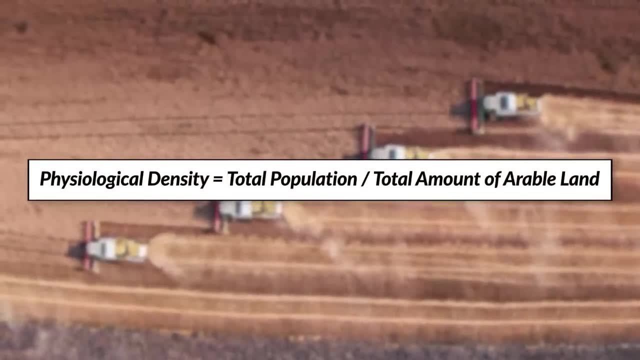 just because a country's arithmetic density is 80 does not mean that each unit of land has 80 people living on it. The next density is the physiological density. To find this density, you're going to take the total population and divide it by the total amount of arable land. Notice, here I said arable. 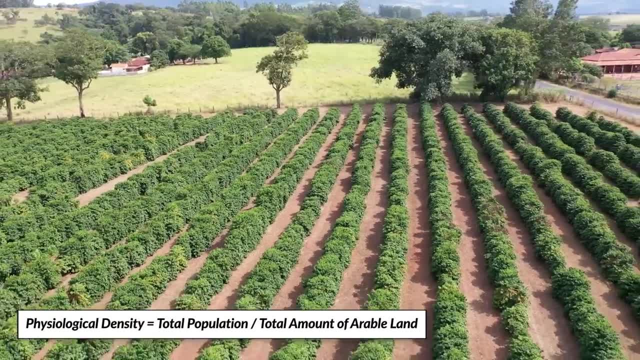 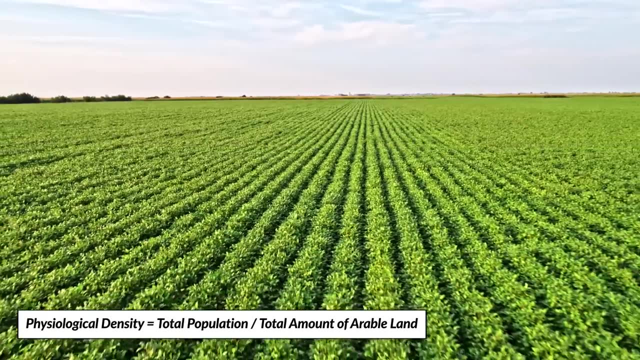 land and not total land area. We are only factoring in land that can produce food. This density shows us how much food we need to produce from one unit of arable land. The higher the number is, the more food we need to produce and the more stress we are going to put on our land Societies. 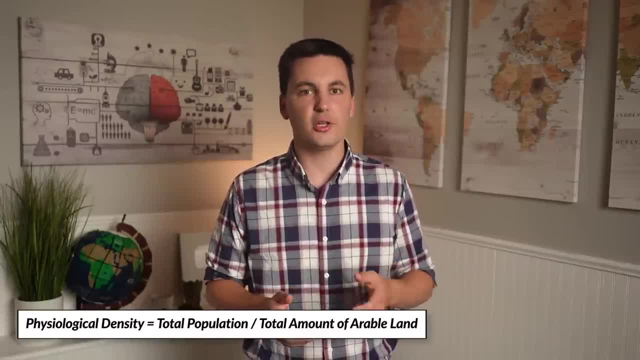 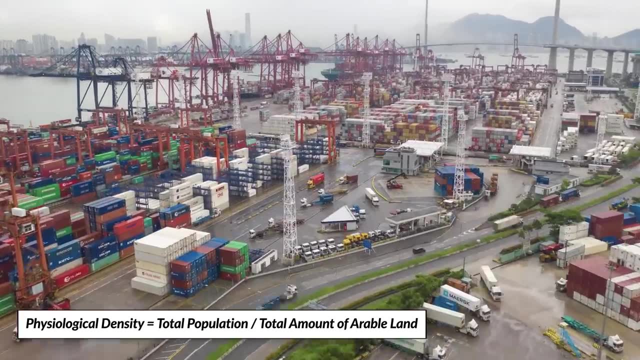 with the physiological density risk desertification and risk destroying their arable land by depleting the nutrients in their soil, which may force them to have to rely on importing food from other societies or countries instead of being able to grow it themselves. The last density is 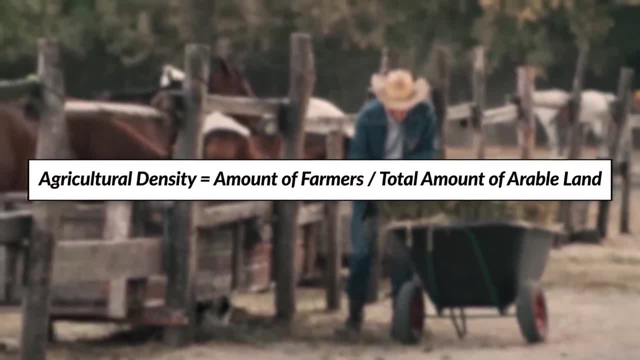 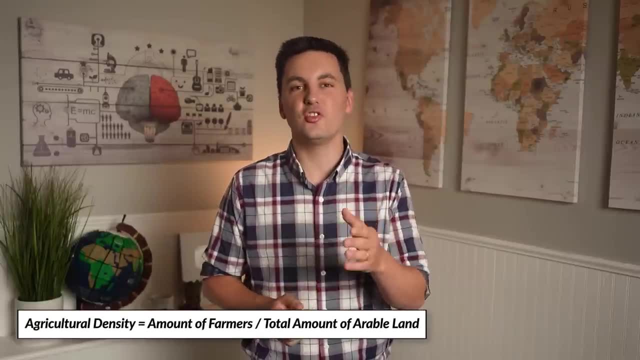 our agricultural density. To find this density, you're going to take the amount of farmers and divide them by the total amount of arable land. This density shows us how advanced the technology is or how efficient a society is at producing food. The higher this number is, the more manual labor a society is using to produce food, For instance. illegal farming provides more doświadment than educational ancestry. Sure money make the difference. response cuts yet. Thanks so much for watching this video And be sure to check out ourographingANDSOCIETYcom for more great textbooks. 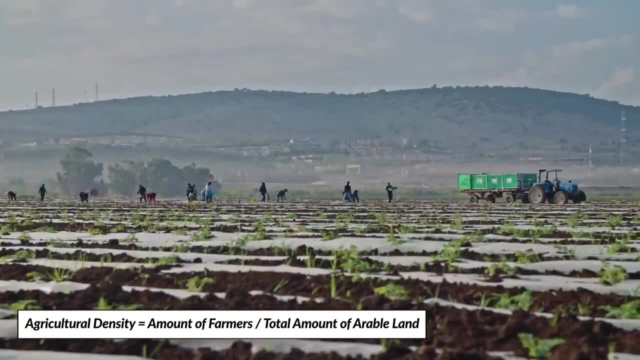 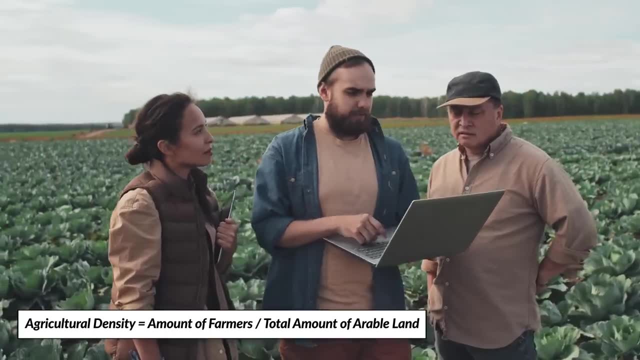 to produce food, which would indicate that there's less technology being used in the field of agriculture or less effective agricultural practices being utilized. The lower this number is, the less human labor is needed, which indicates more efficient agricultural practices. These densities by themselves show different aspects of society, but where the real insight? 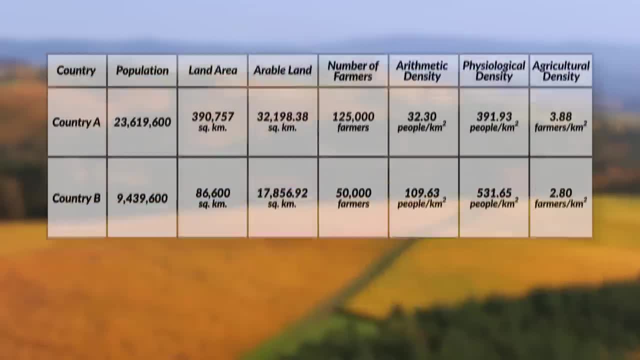 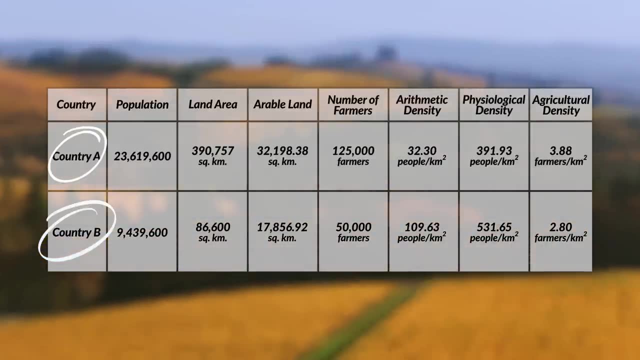 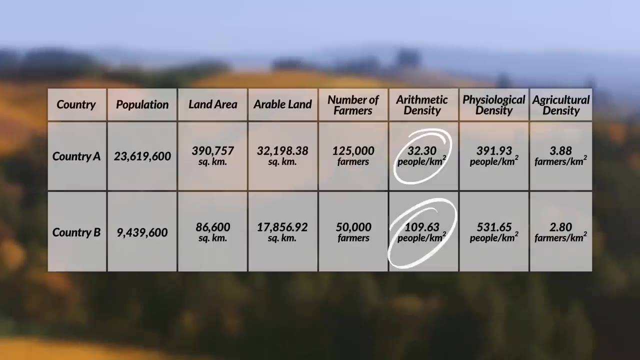 comes from is when you compare them Here. let me show you. Let's say we are comparing two countries. Here we have country A and country B. Right away we can see that country A's population has a lower population density. Their arithmetic density is only 32.3, while country B's arithmetic density is 109.63. 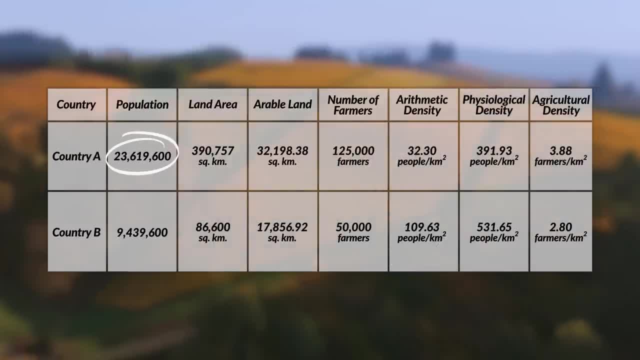 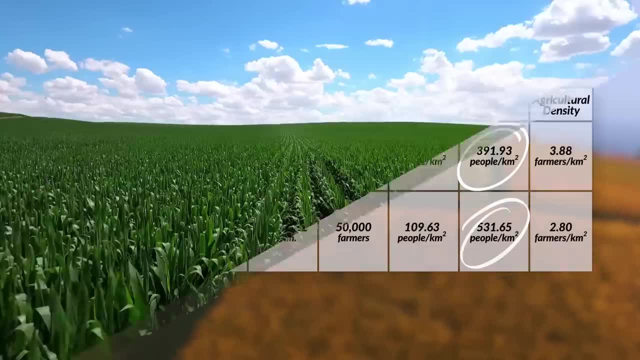 Now we can also notice that country A has a larger population, but if we look at both countries' physiological density, we see that country A's physiological density is lower than country B's. This tells us that country A has more arable land and will have an easier time feeding. 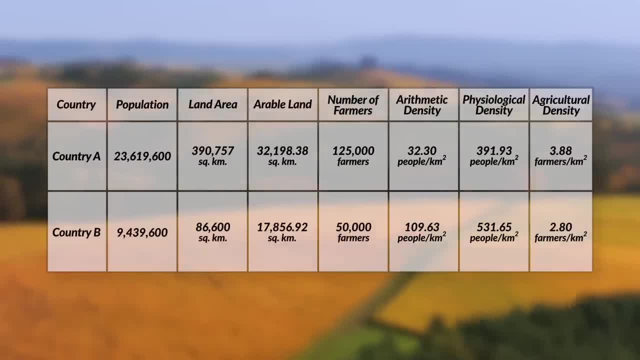 their population. The amount of food that needs to be produced per each unit of land is less for country A than it is for country B, But at the same time we can see that country B's population density is lower than country B's. 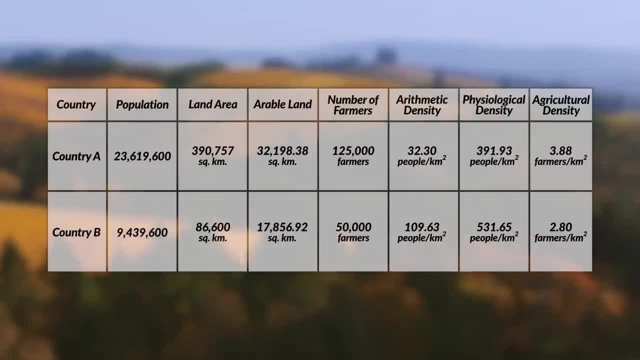 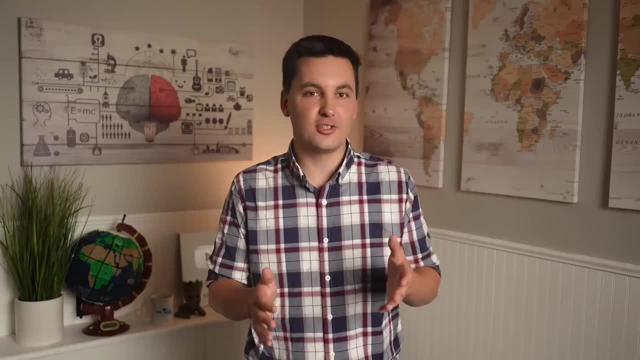 This tells us that country A is less efficient with their agricultural production. Their agricultural density is 3.88, while country B's agricultural density is 2.80. And while that is not a drastic difference, it does show us that country B has slightly.